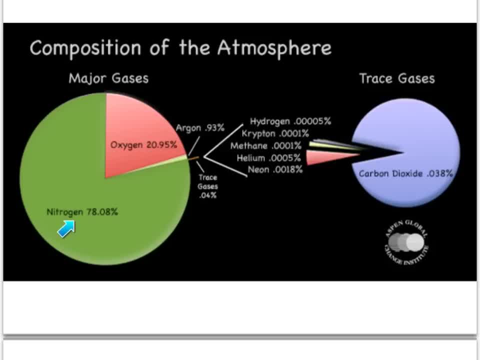 Nitrogen doesn't do anything in our body. We breathe it in, we breathe it out and it just does not affect us. For it to be useful, it actually has to be fixed by bacteria in the soil to be utilized and help make up amino acids and building blocks, parts of organic compounds. 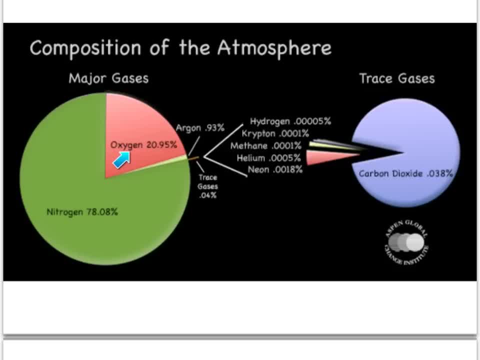 Next most abundant gas in the atmosphere is actually oxygen. Almost 21% of the atmosphere is composed of oxygen, and that's a direct byproduct of photosynthesis, which we'll talk about in our next slide. Past that, There's not a lot left. 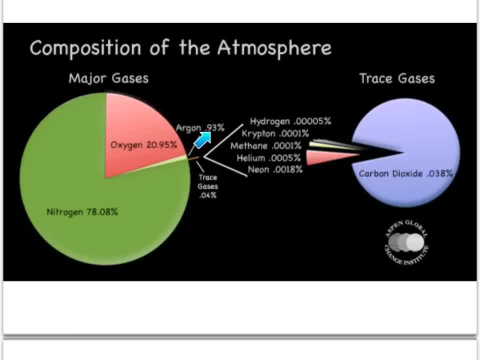 Argon, a little less than 1% Argon, a noble gas, Inert, not doing anything For us anyway. Now all that's left is this really little sliver right there, and that needs to get broken up. 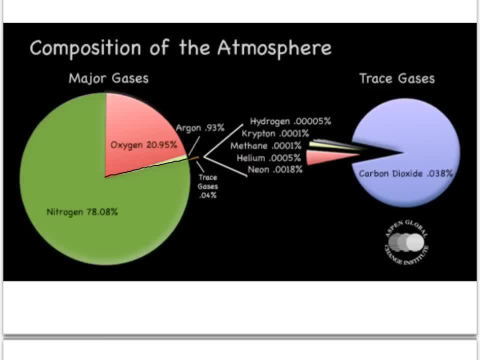 So, if you break that up, we're looking at a really, really small fraction of the atmosphere. now Carbon dioxide, Carbon dioxide- Carbon dioxide makes up 0.038%. That's the fourth most abundant gas in the atmosphere. It's an important one. That is the biggest greenhouse gas, or at least it's the most abundant greenhouse gas, so that plays a huge role in our climate, regulating the climate. 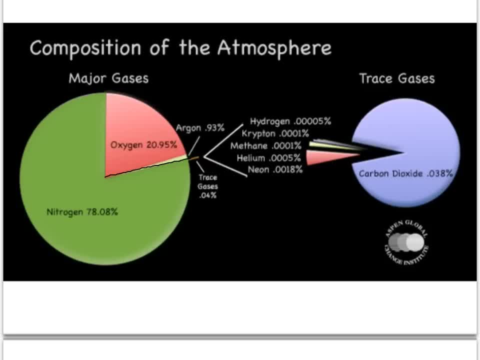 Alright, so those are the four I'm going to test you on, In order from most to the least abundant Nitrogen, oxygen, argon, carbon dioxide, and then I guess we'll go a little further. just at least say these: 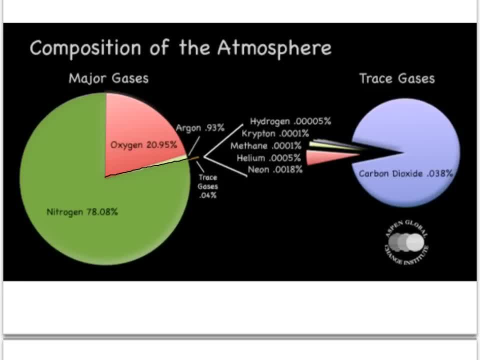 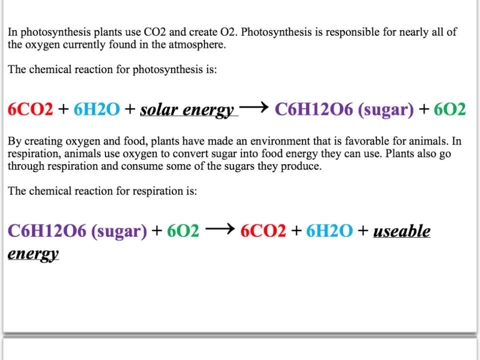 Neon, a noble gas, Helium, methane, CH4, another greenhouse gas, Krypton and hydrogen- all very, very small components of the atmosphere. Alright, so we mentioned that oxygen is the second most abundant gas in the atmosphere, so let's talk about how it got there. 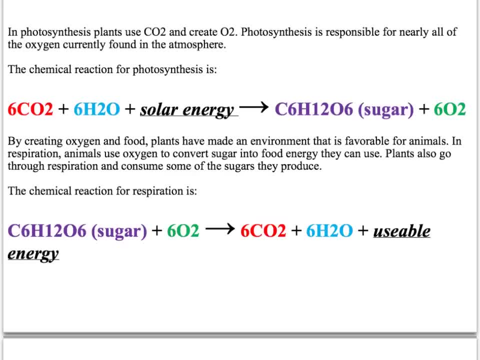 So the chemical reaction that you need to know is photosynthesis. Photosynthesis is where you take carbon dioxide and water, and this really isn't too tricky to remember. Just think you know if you've got a house plant, what is it? 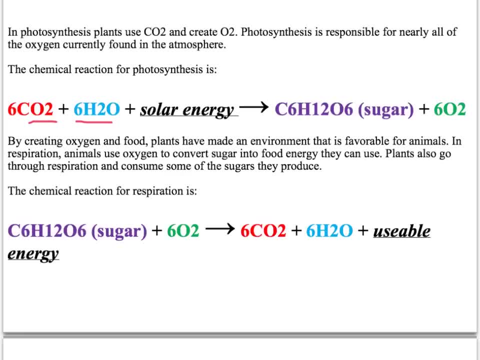 What does the house plant need? right, You need to water the thing to keep it alive, and then it does breathe in what you breathe out. It breathes in carbon dioxide, and it's able to take carbon dioxide and water. It needs energy from the sun, so you've got to put the plant in the light.